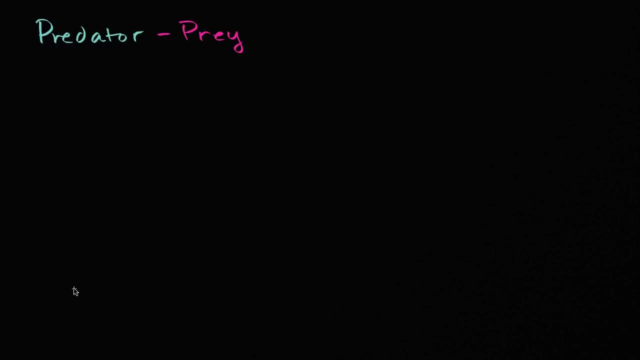 So let's just think about how these populations could interact. Let me draw a little chart here that you're probably familiar with by now, where we show how a population can change over time. So the time the horizontal axis is time, The vertical axis is population. 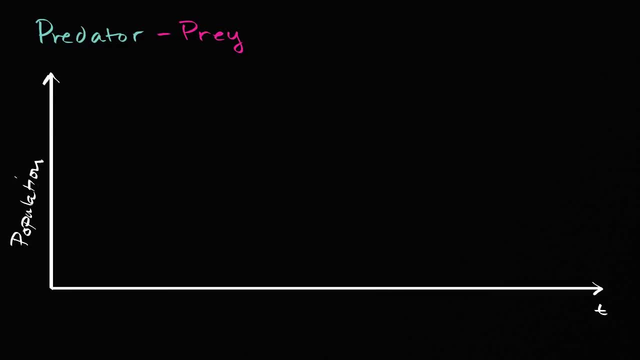 Population. And so let's just in our starting point, let's say that our prey is starting out at a relative relatively high point. Let's say we're right there in time. And let's say, for whatever reason, our predator population is relatively low. 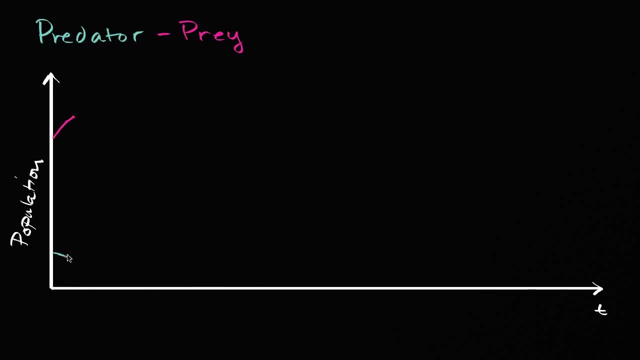 So what do we think is going to happen here? Well, at this point, with a low density of predators, it's going to be much easier for them to find a meal and it's going to be much easier for the prey to get caught. 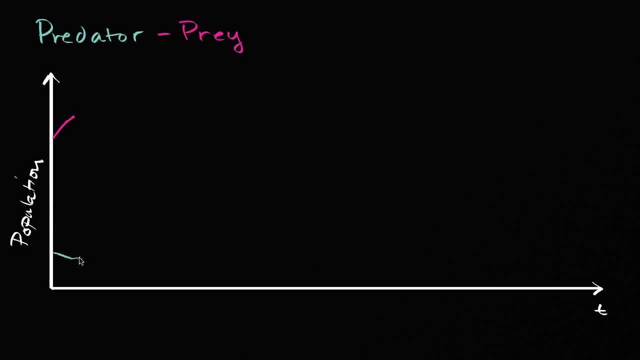 So, since it's more easy, since it's easier for the predators to find a meal, you can imagine their population starting to increase. But what's going to happen as their population is increasing? Well, it's going to be more likely that the prey is going to get caught. 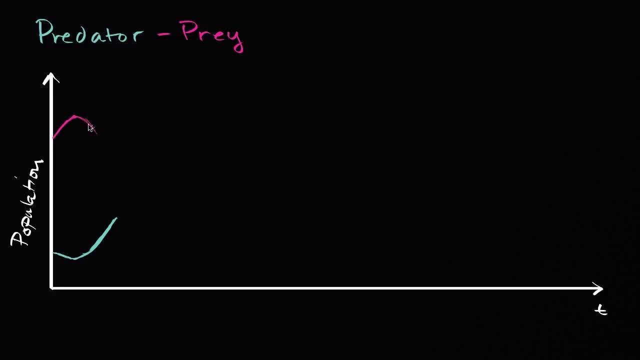 There's going to be more of their hunters around, more of the predators around, So that population is going to start decreasing all the way to a point where, if the population of the prey gets low enough, the predators are going to have 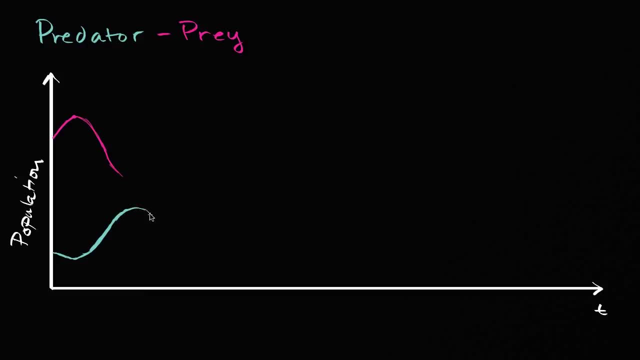 they're going to start having trouble finding food again, and so that their population might start to decrease. And as their population decreases, what's going to happen to the prey? Well then, there's going to be less predators around, so they might be able to their population. 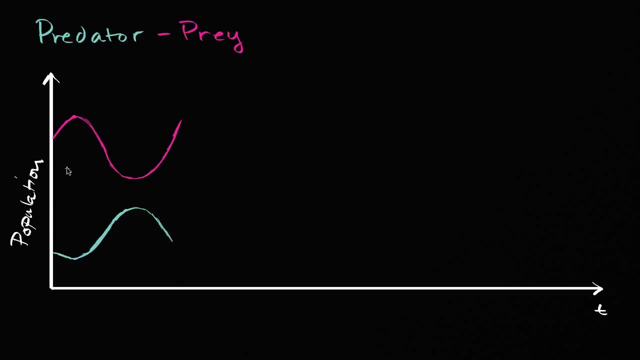 might start to increase. And so I think you see what's happening. The predator and prey, they can kind of form this cyclic interaction with each other, And what I've just drawn, this is often known as the predator-prey cycle, And I just reasoned through that. you could imagine a world. 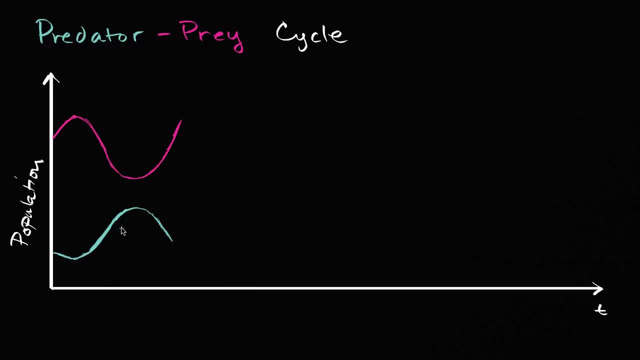 where you could have the cycle between predator and prey populations. but you can also run computer simulations that will show this, And even observational data out in the field also shows this. One of the one of the often-cited examples is interactions between 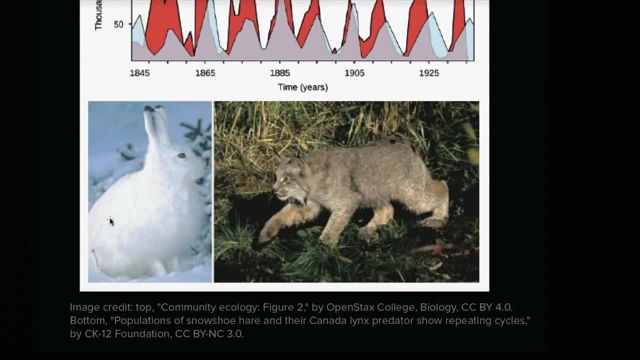 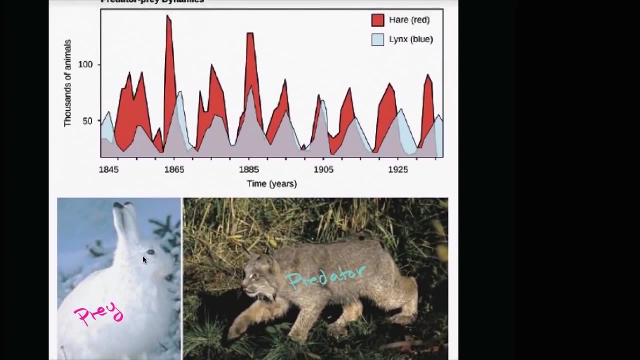 between the snowshoe hare, which would be the prey in this situation, and the Canadian lynx, which would be the predator, the predator in this situation. And you see a very similar cycle to what I just drew, kind of just reasoning through it. 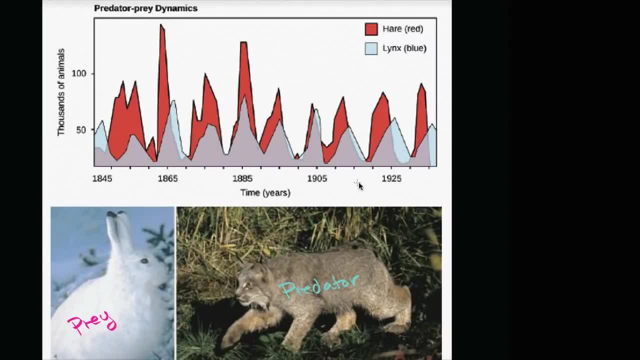 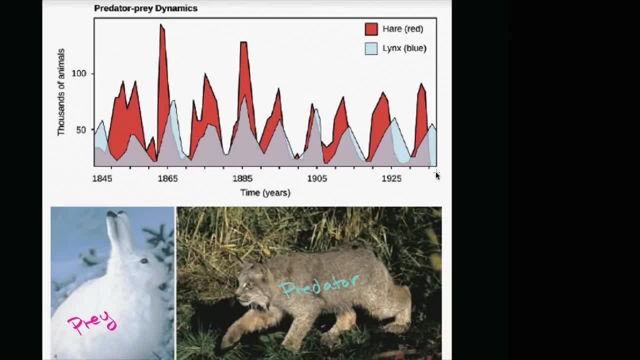 going all the way to the early-mid-1900s, So it's roughly 100 years of data that we're showing And in the vertical axis you have thousands of animals And we're plotting both the population of snowshoe hares. 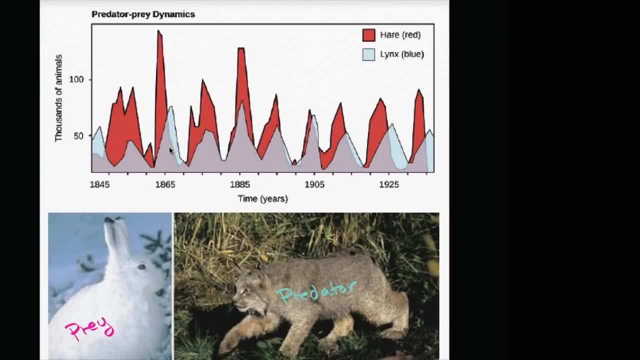 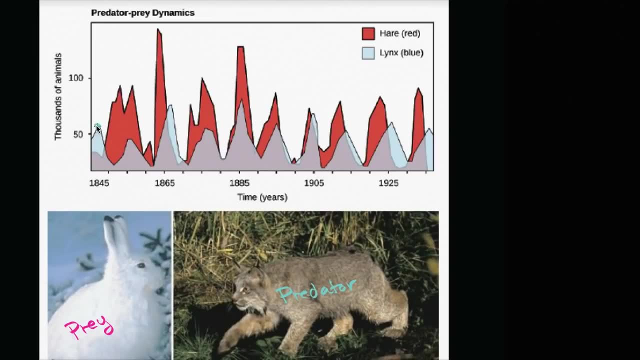 and Canadian lynx in a certain area on this chart And, as you see, when the prey population is high, when the prey population- sorry, when the predator population is high, when we have a lot of the Canadian lynx around, 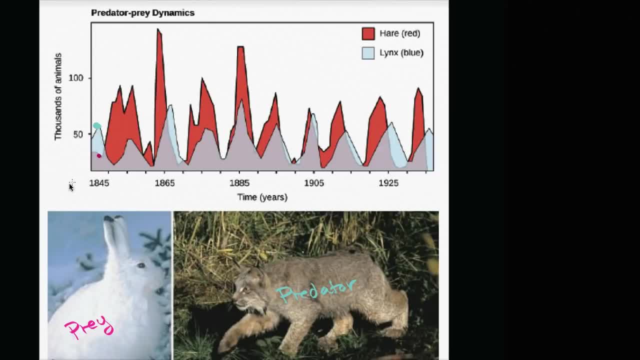 that we see a lower, a lower population of the prey of the hare. But then, as since you have a low population of the food, in this situation, the predator population starts to decrease. So let me draw an arrow here: The predator population starts to decrease. 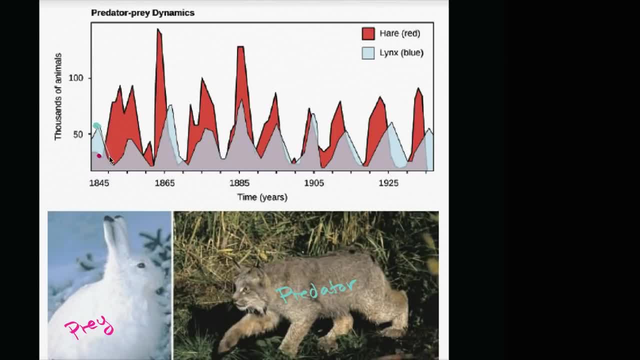 And let me do that same blue color. So the predator population decreases, And as that predator population decreases, well then the prey population increases because there's less folks around to hunt them. So the prey population increases, And you see that the other way around. 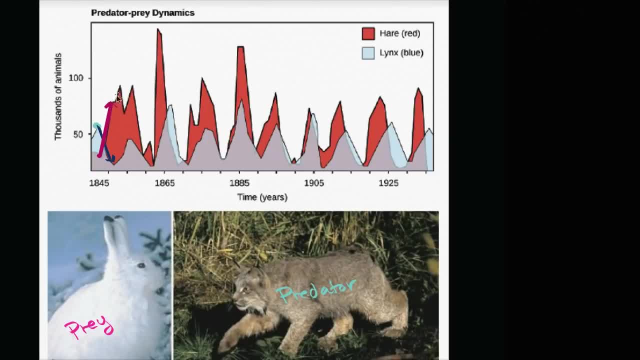 When the prey population is really is, well, maybe we'll show it right over here, and this is real data, so it's not always super clean. But when the prey population is really really high and the predator population is relatively low, well then. 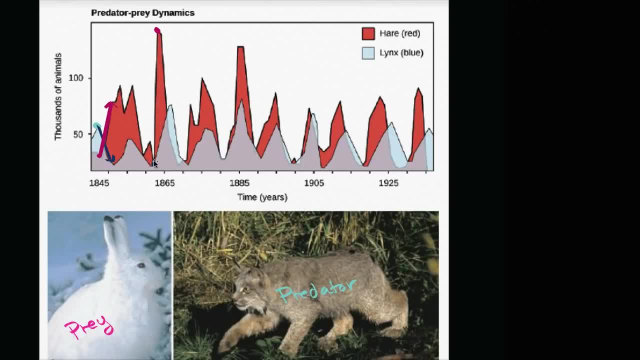 the predators say, hey, it's really easy for us to find meals right now. That was kind of that starting point in when I just was reasoning through it, And so their population starts. whoops. what did I do There? there, let me make sure.